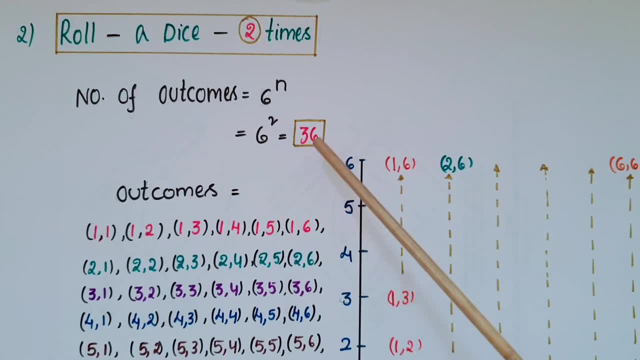 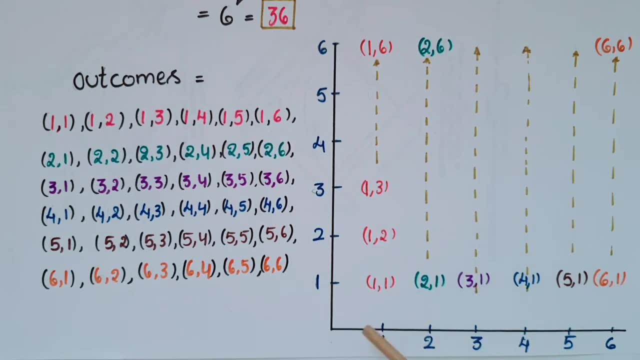 2 is two times, So that is 36.. So now I am going to tell how to write these 36 outcomes. So for this, draw a horizontal line and show 1,, 2,, 3,, 4,, 5,, 6 and draw a vertical line. 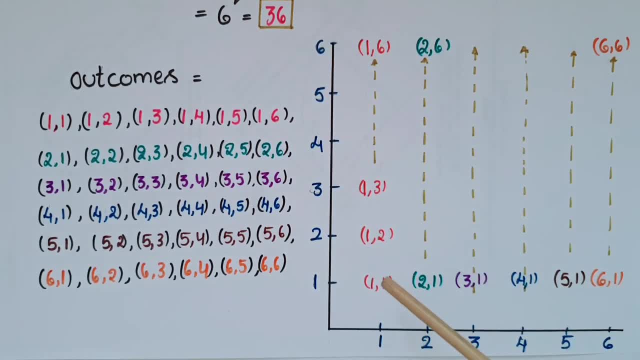 like this and show 1,, 2,, 3,, 4,, 5, 6 and start writing outcomes like this: 1, 1, 1, 2 until 1, 6.. So right here: 1, 1, 2, 1, 6 and second: 2, 1, 2, 2, 6.. So 2, 1, 2, 2, 6 and 3, 1, 2,, 3, 6, like this: 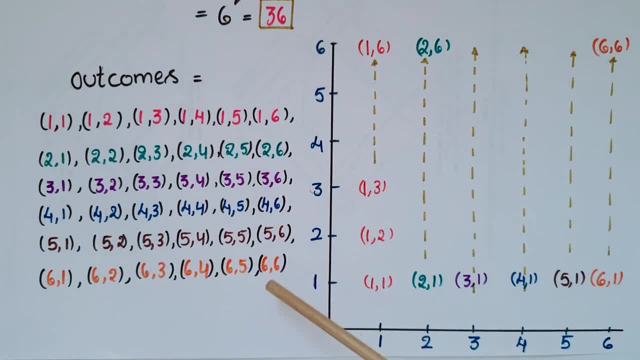 4, 1, 2, 4, 6, 5, 1, 2, 5, 6 and 6, 1, 2, 6, 6.. So these are total 36 outcomes for roll a dice two times. 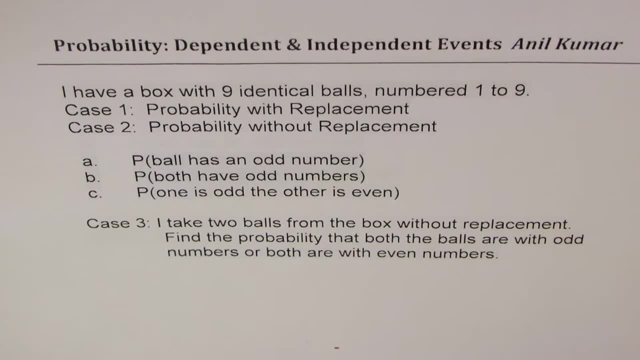 I'm Anil Kumar, sharing with you a video on probability. We may also touch upon the terms like dependent and independent events. Let me first thank my subscriber, Irum, for sharing this question, and I hope the solution will help many others. The question here is: I have a box with